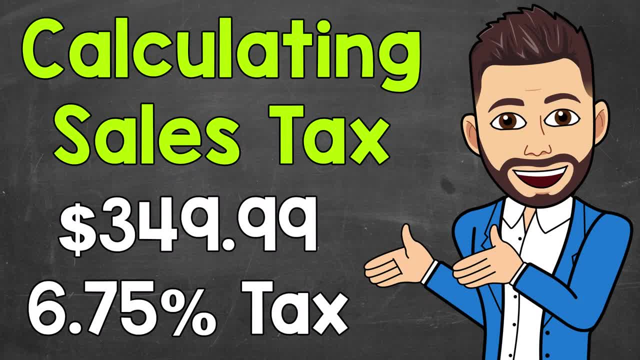 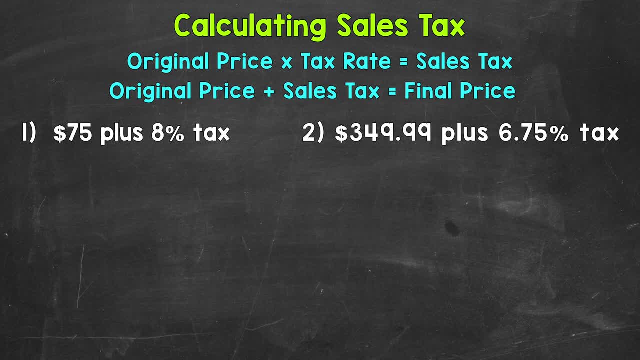 Welcome to Math with Mr J. In this video I'm going to cover how to calculate sales tax and then the final price with that tax included. Let's jump into our examples and see exactly how we do this, Starting with number one, where we have a price of $75 and then a sales tax rate of 8%. 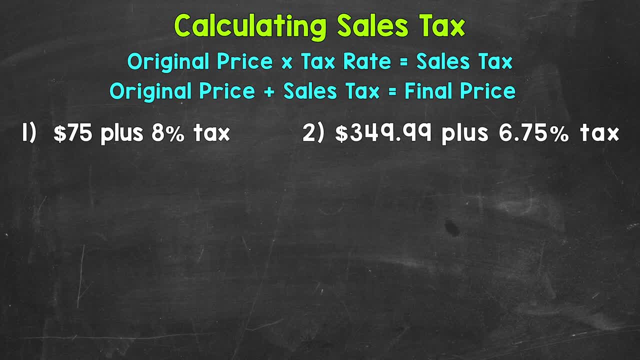 Now I do want to mention that sales tax rates vary by country and state, and then there can be local taxes that are included as well. This video does not cover a specific location sales tax. These are general numbers being used to show how to calculate sales tax. So the first thing that 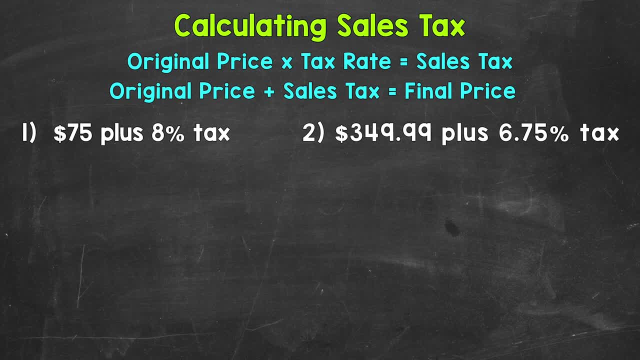 we want to do is to calculate how much sales tax we will be paying. We do this by multiplying the price by the number of sales tax we will be paying. We do this by multiplying the price by the tax rate. The tax rate is going to be in the form of a percent. We want to get this percent. 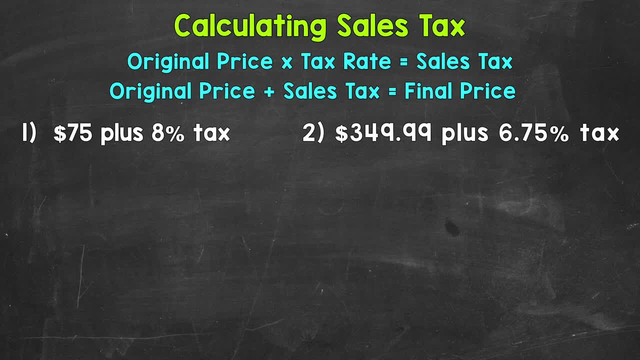 to decimal form. Percent means per 100. So we divide the percent by 100 to convert it to a decimal. We can do this by simply moving the decimal twice to the left. So percent to decimal. move the decimal twice to the left, That gives us a decimal equivalent to the percent. 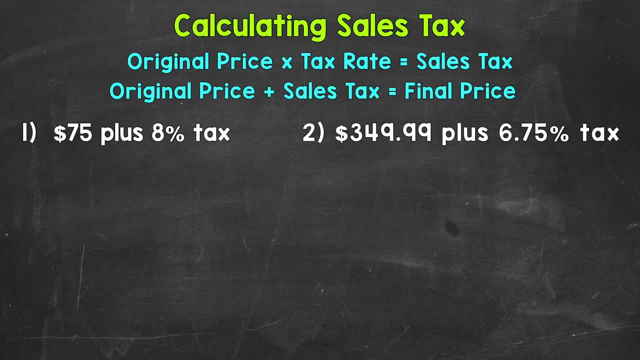 So for number one we have 8%. Let's move that decimal twice to the left. I'm going to rewrite 8% underneath here, so I have enough room Now for a whole number. the decimal comes after a whole number, So it's right here for 8% Once, twice to the left. So we have 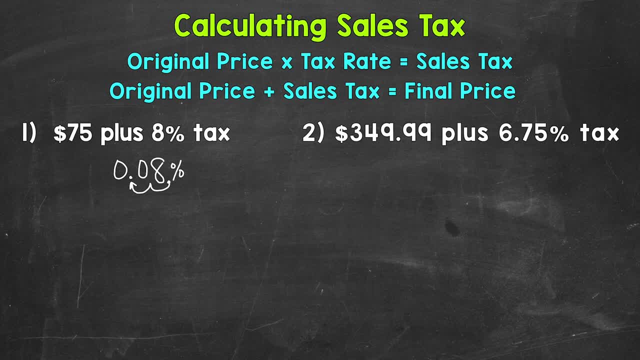 0.08 for decimal form there. So we need to take our original price of $75.. $75 here and multiply that by 0.08.. Now if you are using a calculator with a percent button, you can also do $75 times 8%. So you can leave it in percent form. 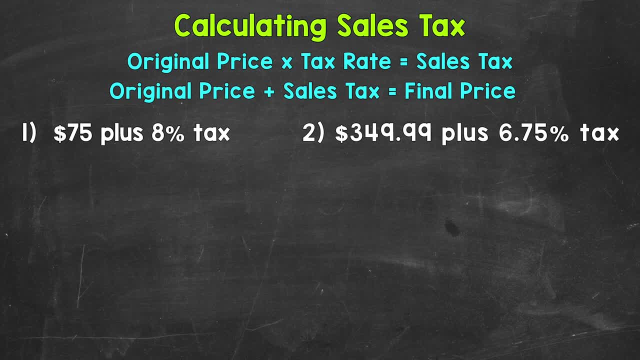 we want to do is to calculate how much sales tax we will be paying. We do this by multiplying the price by the number of sales tax we will be paying. We do this by multiplying the price by the tax rate. The tax rate is going to be in the form of a percent. We want to get this percent. 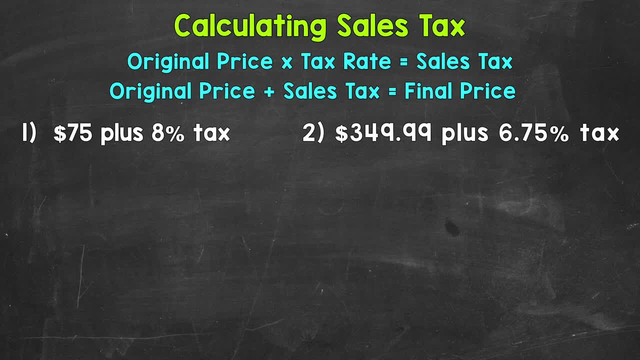 to decimal form. Percent means per 100. So we divide the percent by 100 to convert it to a decimal. We can do this by simply moving the decimal twice to the left. So percent to decimal. move the decimal twice to the left, That gives us a decimal equivalent to the percent. 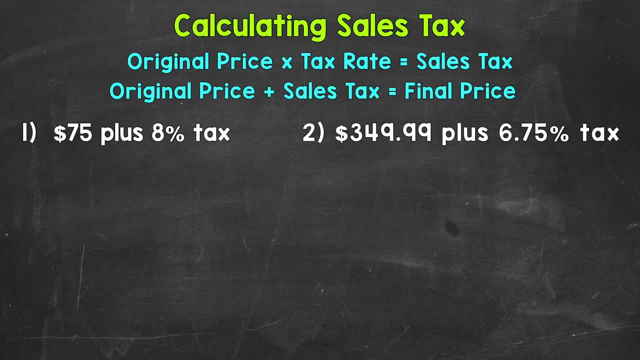 So for number one we have 8%. Let's move that decimal twice to the left. I'm going to rewrite 8% underneath here, so I have enough room Now for a whole number. the decimal comes after a whole number, So it's right here for 8% Once, twice to the left. So we have 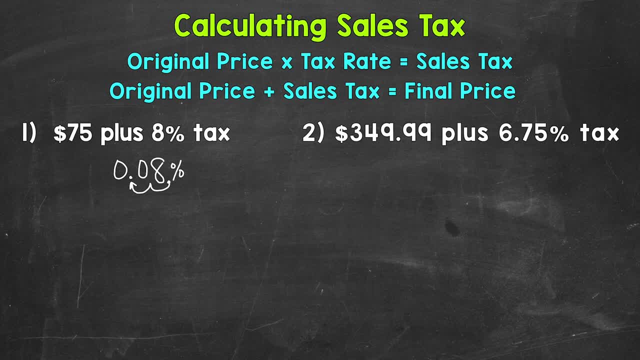 0.08 for decimal form there. So we need to take our original price of $75.. $75 here and multiply that by 0.08.. Now if you are using a calculator with a percent button, you can also do $75 times 8%. So you can leave it in percent form. 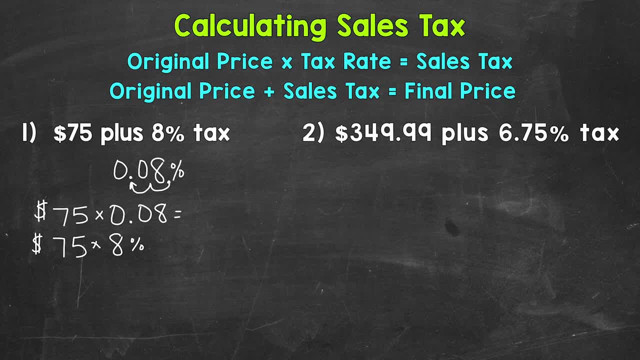 just make sure you hit that percent button. Do not do 75 times 8.. So either one of those will give us the correct answer as far as how much we are paying in sales tax. So 75 times 0.08, that's going to give us $6.. Now, 75 times 8%, that gives us the same. 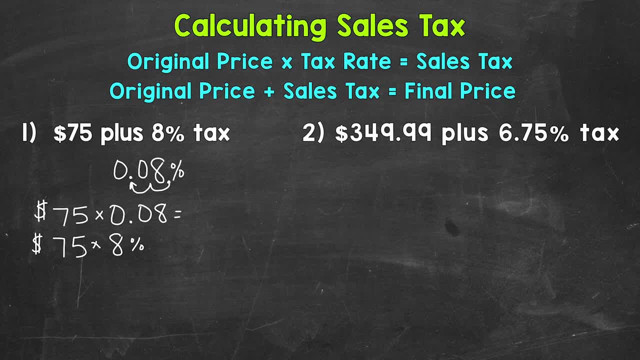 just make sure you hit that percent button. Do not do 75 times 8.. So either one of those will give us the correct answer as far as how much we are paying in sales tax. So 75 times 0.08, that's going to give us $6.. Now, 75 times 8%, that gives us the same. 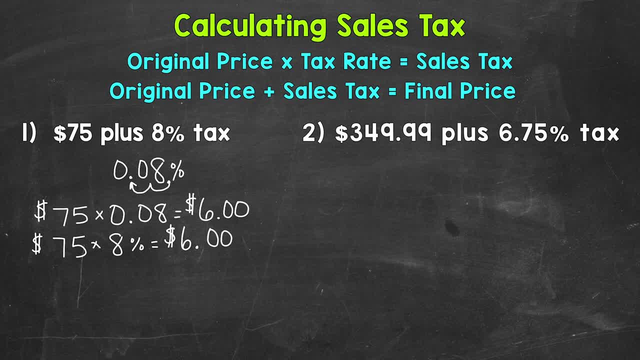 answer of $6.. So that's how much we are going to pay in tax. So once we have that information, we take our original price and add that sales tax to give us our final price. Make sure you add that sales tax So we have- I'll write this out by hand- We have $75. 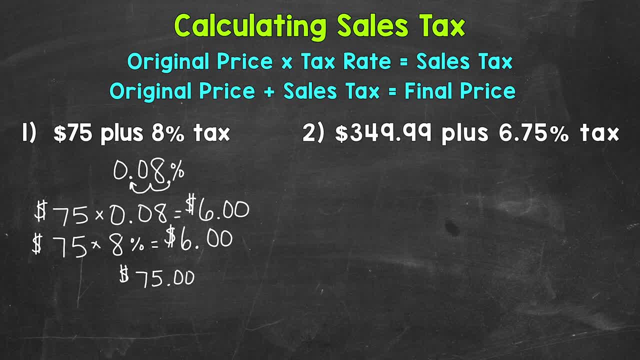 plus $6.. So that's going to give us a total price, with tax included, of $81.. Let's move on to number two, where we have $349.99 for our price and then a sales tax rate of 6.75%. Let's convert that sales tax rate to $6.75.. So that's going to give us a total price. 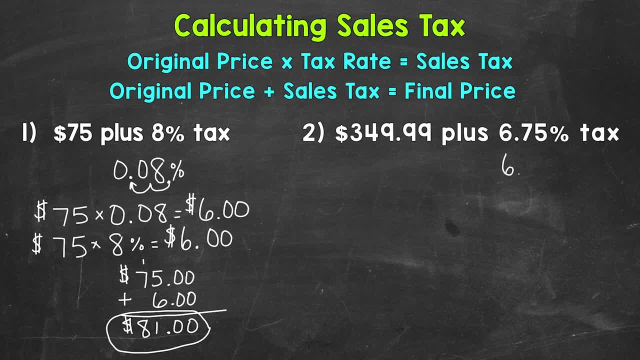 of $349.99.. I'm going to go ahead and do a decimal: Move the decimal twice to the left, So I'm going to rewrite this underneath here so we have enough room- And move it once twice, So we have .0675 for our decimal. So let's multiply that by our. 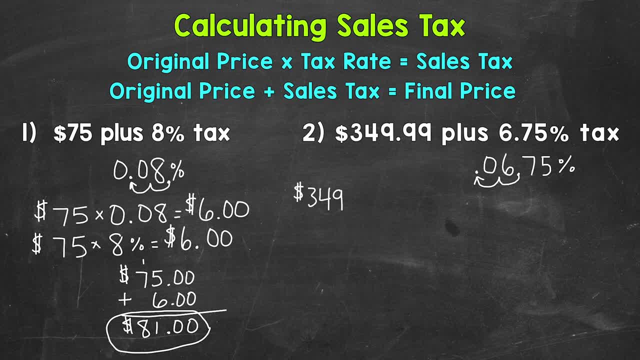 original price of $349.99.. decimal form of 0.0675.. Now we can also do this using the percent button on a calculator, So I'll write that out just to be clear here. So we can do $349.99 times 6.75 percent, And these are both. 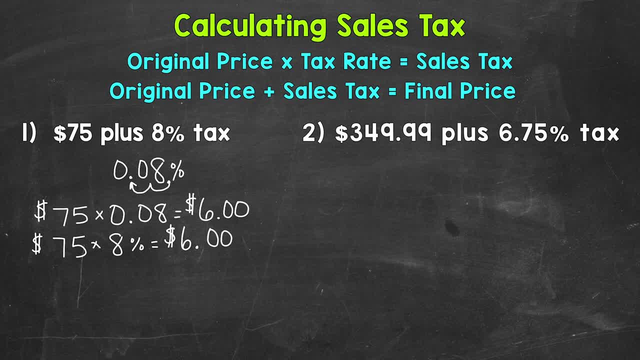 answer of $6.. So that's how much we are going to pay in tax. So once we have that information, we take our original price and add that sales tax to give us our final price. Make sure you add that sales tax So we have- I'll write this out by hand- We have $75. 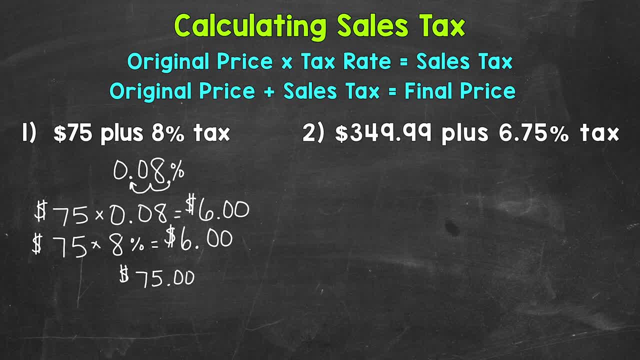 plus $6.. So that's going to give us a total price, with tax included, of $81.. Let's move on to number two, where we have $349.99 for our price and then a sales tax rate of 6.75%. Let's convert that sales tax rate to $6.75.. So that's going to give us a total price. 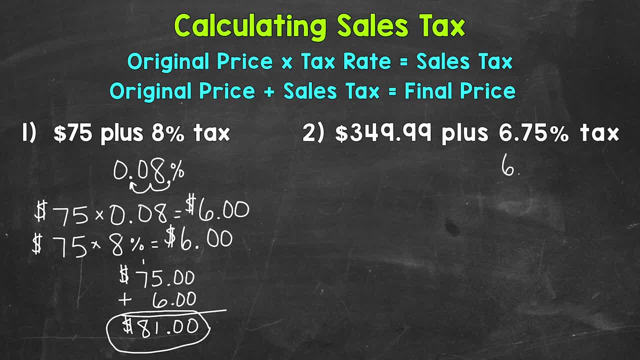 of $人民불가 $135.99 for our price. So it is $3.95.. So we have $39.99.. I'm going to rewrite this underneath here so we have enough room, And move it once twice so we have. 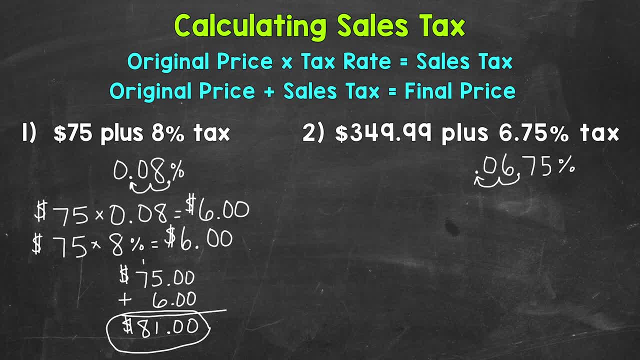 0.0675 for our decimal. So let's multiply that by our original price of $349.99.. So there we go, Excellent, Excellent. Let's say we have $174.99, and we're going to put this down. So let's just do a decimal. 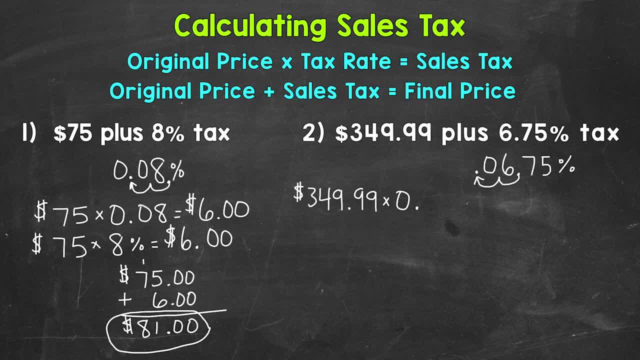 Let's say we have $174.99.. So if we look at the difference, we can see that our sales tax rate is $2.89.. decimal form of 0.0675.. Now we can also do this using the percent button on a calculator. So I'll. 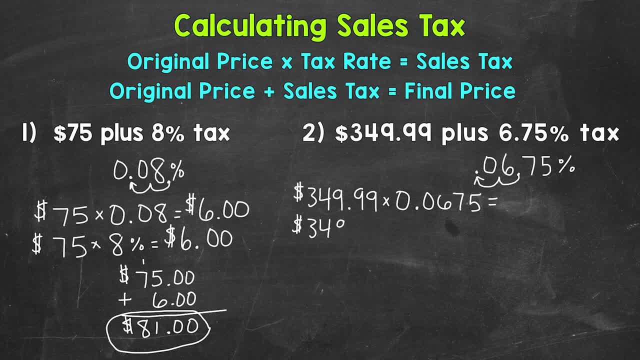 write that out just to be clear here. So we can do $349.99 times 6.75 percent, And these are both going to give us the correct answer of now. for this one we get a fairly long decimal, So 624325.. 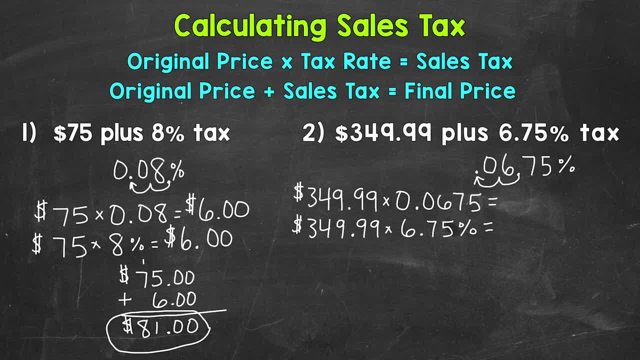 going to give us the correct answer of now. for this one we get a fairly long decimal, So 624325.. I'll write that out for both here. Now we are working with money, So money always goes to the hundredths place. So if you get a long decimal like this, we round to the hundredths. 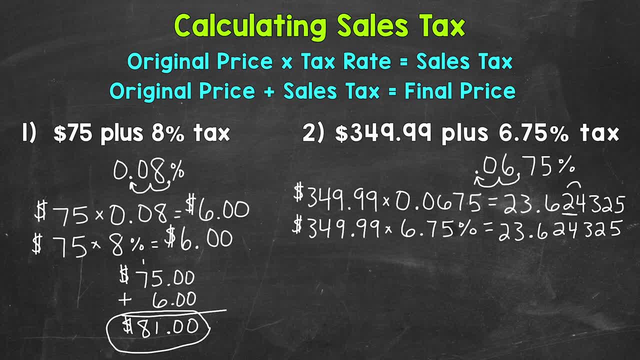 place. So this two here in the hundredths look next door and we stay the same. So this is going to round to- let me rewrite it- underneath $23.62.. So that's going to be how much we are going to pay. 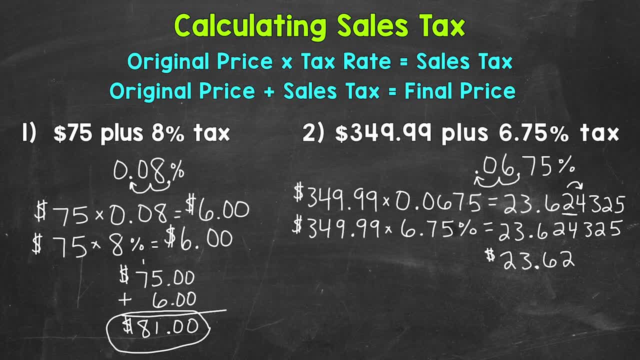 in sales tax. Once we have that information, we add it to our original price. I'll write this out. So we have $349.. $349.99 plus $23.62.. So let's add here: 9 plus 2 is 11.. 1 plus 9 is 10 plus 6 is 16.. Bring our decimal. 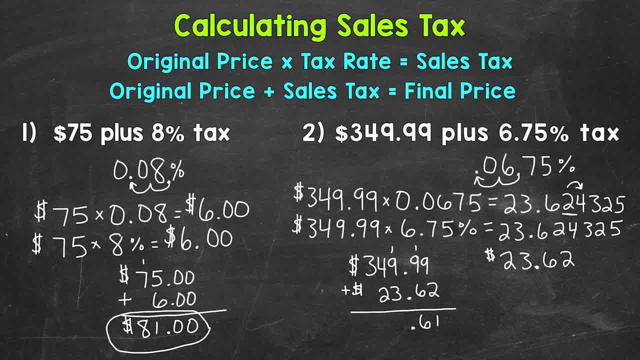 straight down: 1 plus 9 is 10, plus 3 is 13.. 1 plus 4 is 5, plus 5 is 6.. So we have $349.99 plus $23.62.. Plus 2 is 7.. And then we have a 3 in the hundredths place. So our final price with sales tax included. 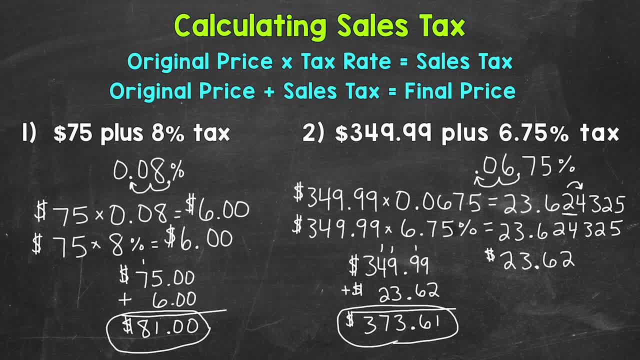 is going to be $373.61.. So there you have it. There's how you calculate sales tax. Take that original price and multiply it by the tax rate, either in decimal form or use the percent button on a calculator. That's going to get you $349.99.. So that's how you calculate sales tax. 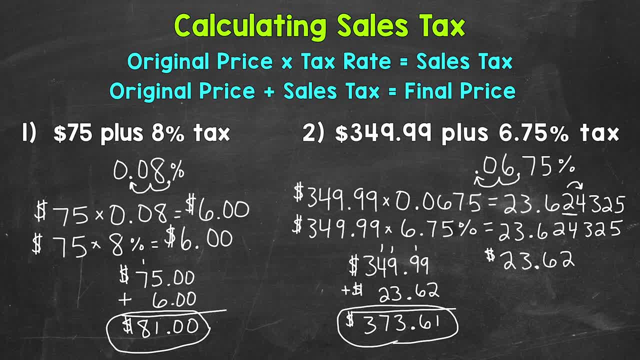 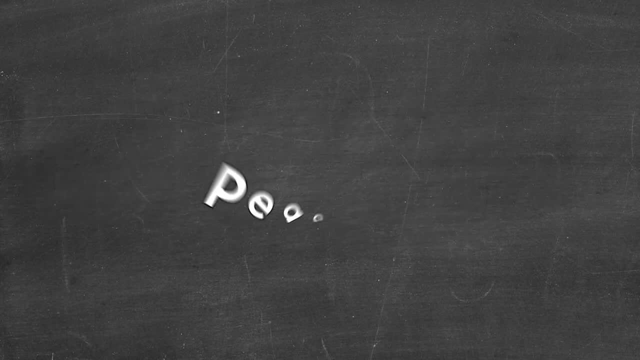 Once you have that information, you take the original price and add that sales tax to get the final price. I hope that helped. Thanks so much for watching. Until next time, peace.